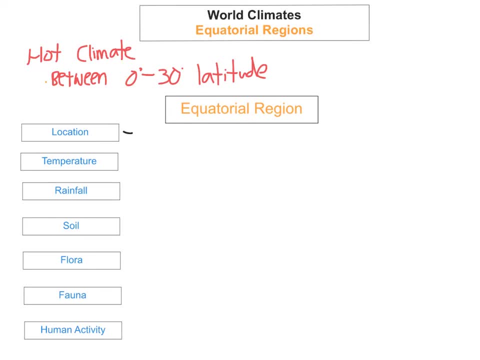 So the first one location: where will you find equatorial regions? Well, you'll find them 8 degrees north and 8 degrees south of the equator. An example of a country that you'll find this climate is Indonesia. So Indonesia is an example of a country that will experience this climate. 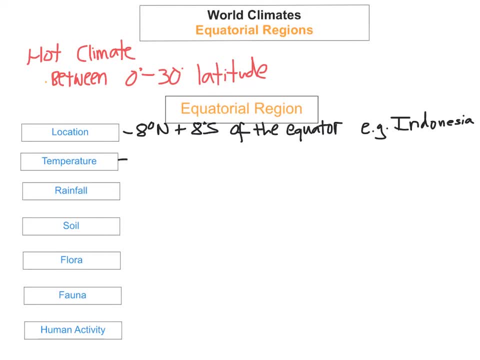 Temperature. Okay, so what is a temperature? The average daily temperature is 27 to 28 degrees. So average temperature absolution Is 27 to 28 degrees Celsius, So that is 4 degrees in the on the globe Rainfall. They have very high levels of humidity, okay, and 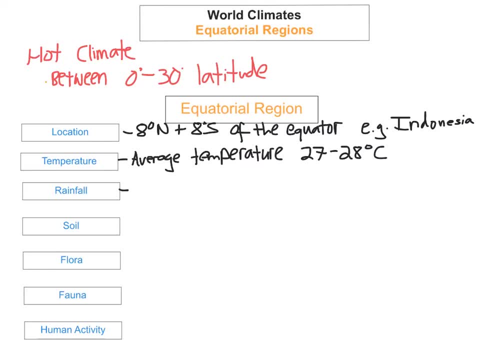 because a lot of the water, the moisture, evaporates away, they get a lot of convectional rainfall, So convectional rainfall, And they can experience thunderstorms for many days and this is because of the high levels of evaporation that leads to the convection rainfall and they'll get 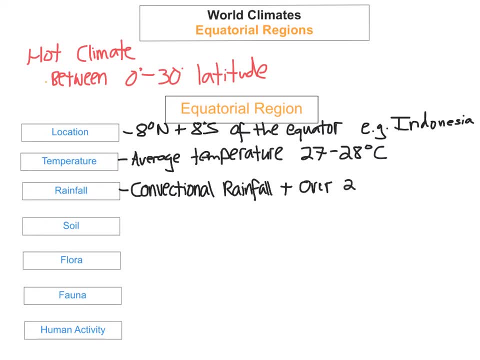 over 2,000 millimeters of rain annually. The next one is a soil type and they have a tropical red soils. So tropical red soils- And, as we know from studying soils, tropical red soils- are not very fertile, which results in intense weathering of the soils and the rocks and 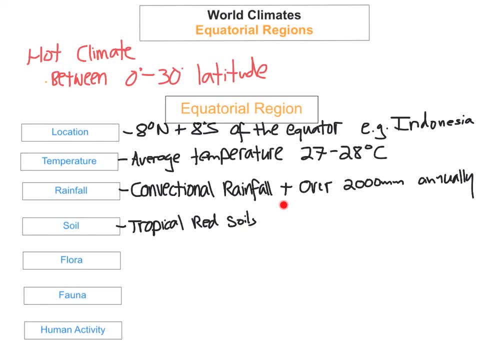 when you get this very heavy convectional rainfall and because of the amount of rainfall that they actually get, they get a lot of leaching, which leads to a lot of the nutrients from the soil being leached and washed down from the A horizon to the B horizon and therefore 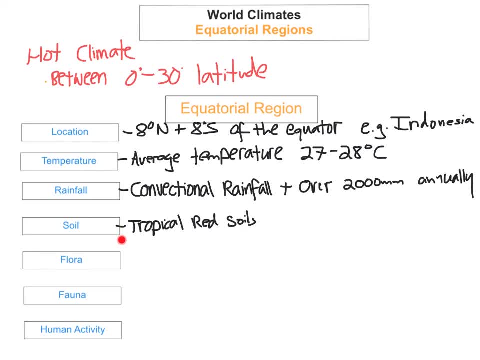 it makes it really hard to grow vegetation and this is a huge problem in equatorial regions. At equatorial regions, because of the amount of rainfall that they get, the flora is most of the vegetation is going to be rainforests or jungle. 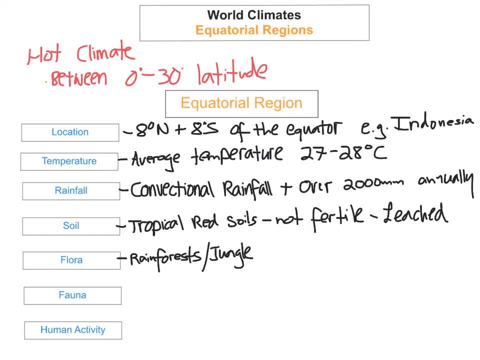 So rainforests are dense hard tree woods such as mahogany, and the canopy roof is formed by a topsoil. The topsoil is the tops of the trees, and the trees block out lots of sunshine for the areas underneath the trees, so the forest floor doesn't receive that much light. 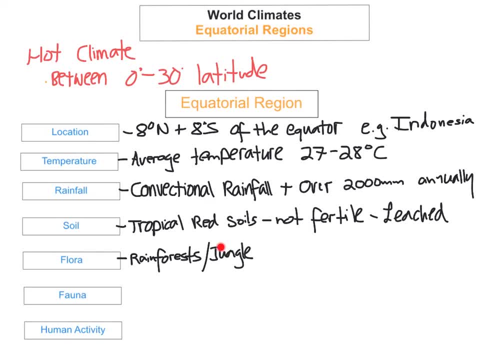 So the taller trees in the emergent layer stick up to above the canopy because they want to try and get some sunshine, and the area between the canopy and the forest floor is the understory and they don't receive much light at all. The fauna, so the different animals and the species. these include, like monkeys, 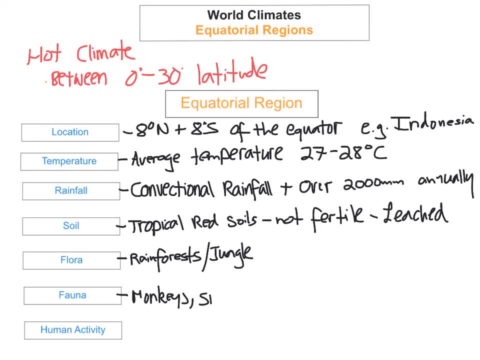 snakes, parrots and butterflies. And the last one we're going to look at is human activity, and one of the things that is becoming prominent in the last few years is deforestation of the rainforests, Which is leading to many, many problems for humans and for the traditional people. that 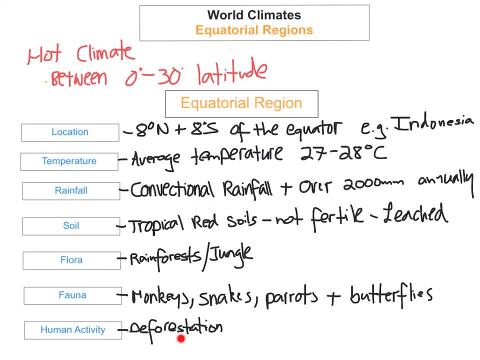 actually live within the rainforests, so the tribal people. Large areas of the rainforests are being cleared because of deforestation to make room for cattle, ranching, mining, roads for logging, etc. And trees are burnt to clear these areas and cut down to sell on the timber.